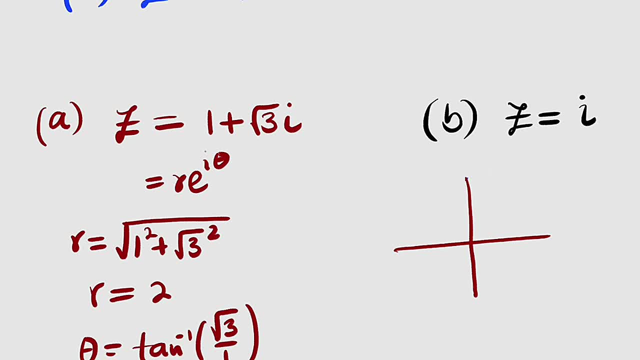 do this is to transform this complex number into its exponential form. Let's take the other one. All right, here is the second one. z is only equal to i, so the real part is missing. So if you should construct this, you know it is going to lie on y-axis here, right? Therefore, the angles of tender is what? 90 degrees, or pi divided by two? And what about the radius? You know, the coefficient of i is just one, so the distance here is one. 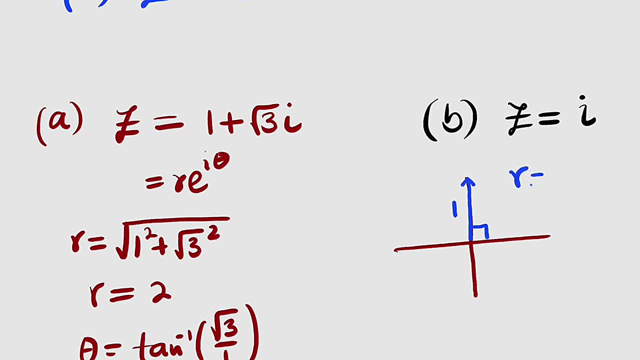 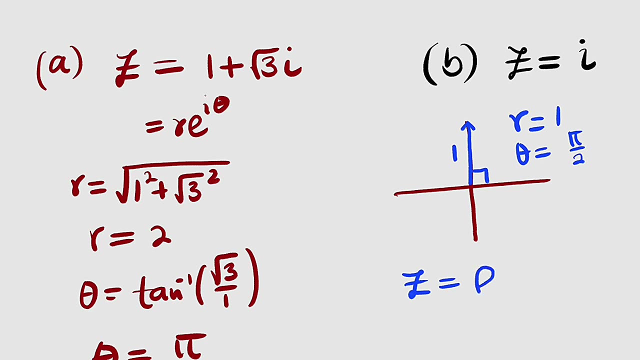 because r is the distance, So r is equal to one and r theta is equal to 90 degrees, or pi divided by two, And so we can transform this complex number into z equal to r, which is one. we don't have to write it. 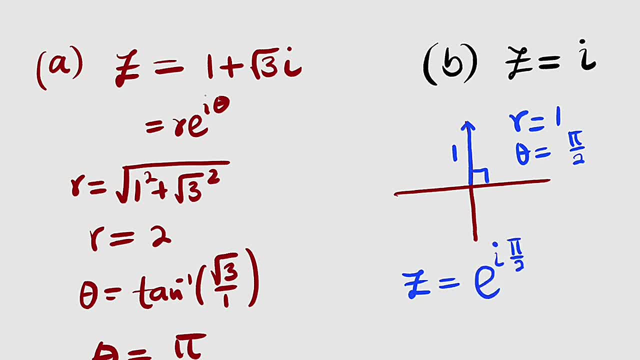 e to the i theta is what pi divided by two, And from this you'll be able to transform it back into this. it's all the same. So now let us take problem number three. All right, here is problem number three. 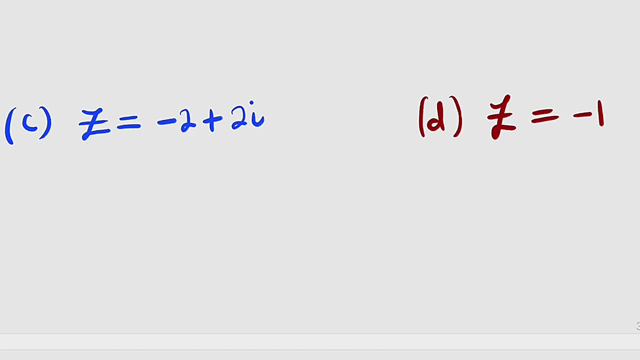 You can see z equal to negative two plus two i. I think this is in the second quadrant, which is less than 180.. So if we should take reference from the first quadrant, we are going to subtract whatever we obtain from 180 degrees. 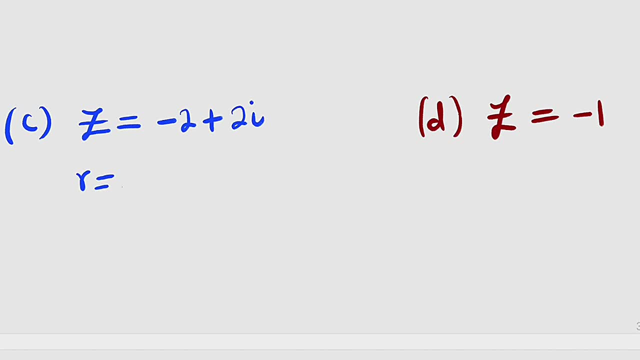 So let's start by finding the radius r equal to the square root of negative two squared plus two. Negative two squared is four, and two squared is four. Four plus four is eight, And square root of eight is what Two root two. 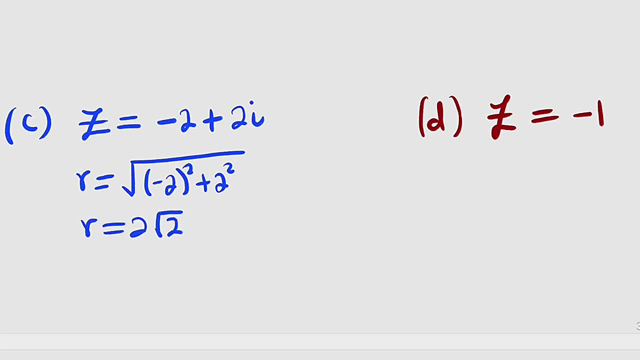 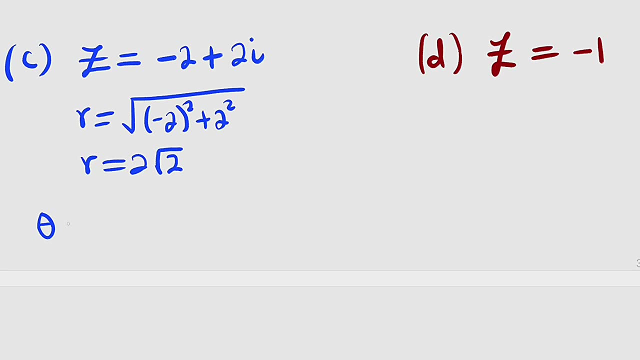 Therefore, r is equal to two root two. And what about the angle? Remember, this is in the second quadrant, which is less than 180.. Therefore, whatever we obtain, we have to take it away from pi, which is 180.. 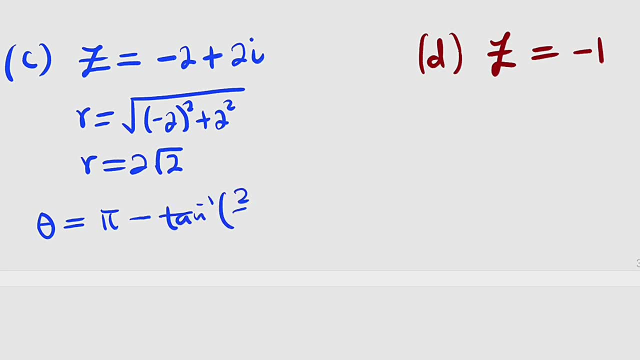 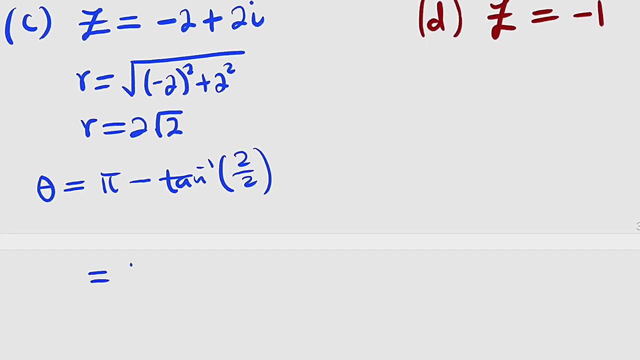 Then turn inverse of what Two divided by two. We are taking everything positive, because in the first quadrant everything is positive. Two divided by two is one. Turn inverse of one is pi divided by four. So our angle is now equal to pi minus pi divided by four.